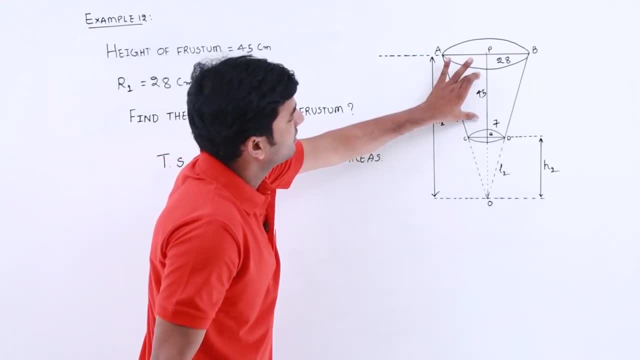 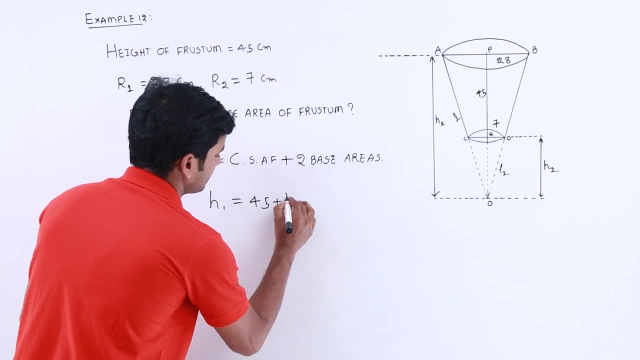 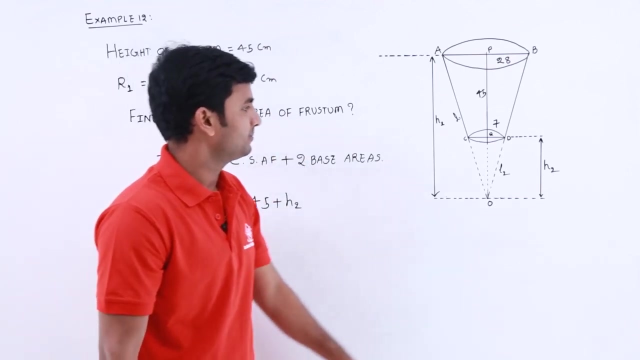 H1 is equal to height of this first term plus the extended portion cone height, that is, 45 plus H2.. Here we don't know the value of H1 and H2. But if you observe carefully this diagram, triangle OQD and triangle OPB are similar. 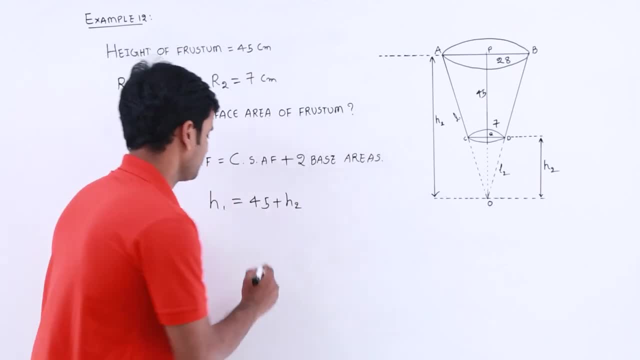 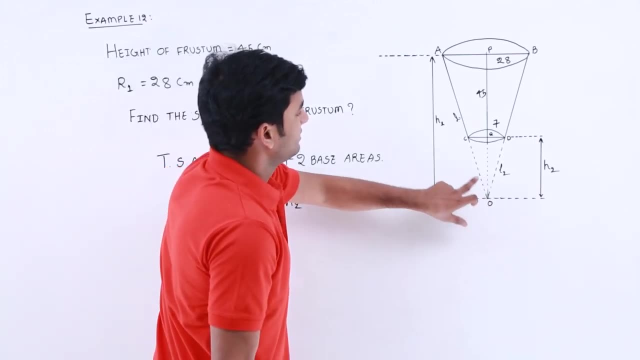 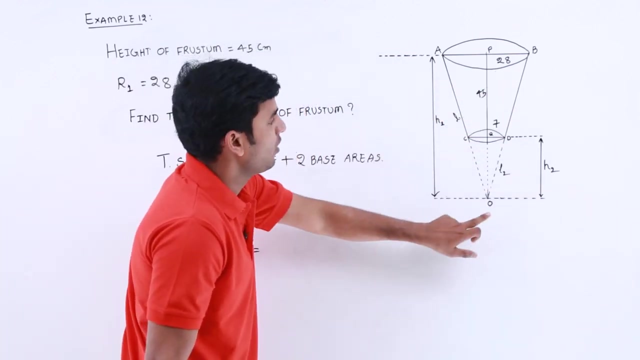 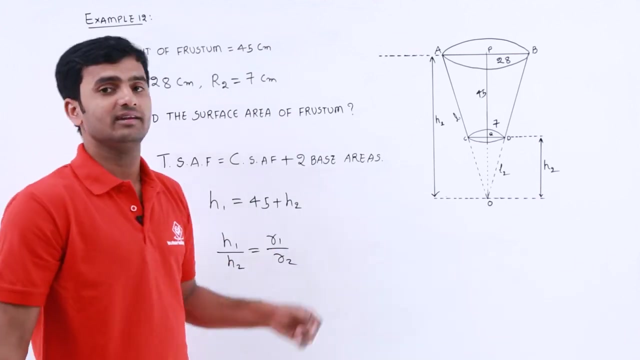 So based on similar triangle concepts, we can find out that that is H1 by H2 is equal to this: H1 is one side of triangle OPB and this H2 is one side of triangle OQD. That will be R1 by R2.. So in similar triangle the respective side ratio will be equal. 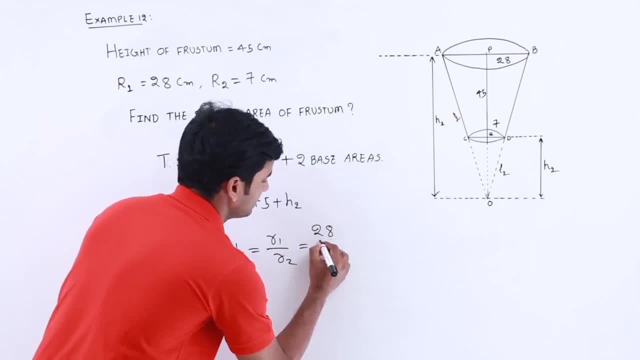 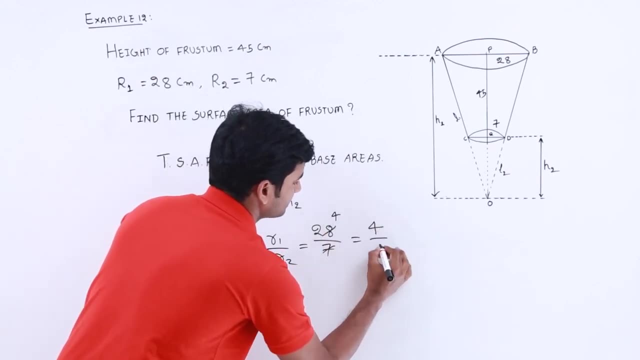 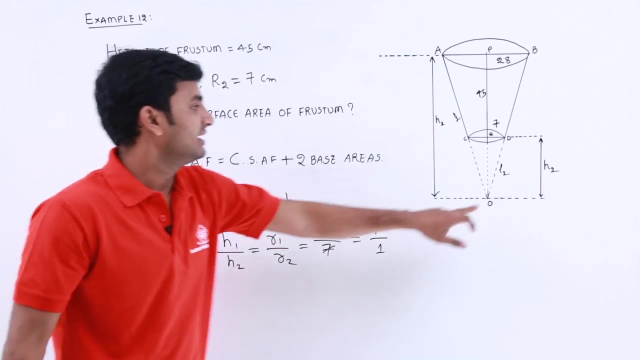 So here we know: R1, that is 28, and R2, that is 7.. So 7 forger. So it will become 4 by 1.. Here the H1 is complete height of this cone and H2 is extended cone height. 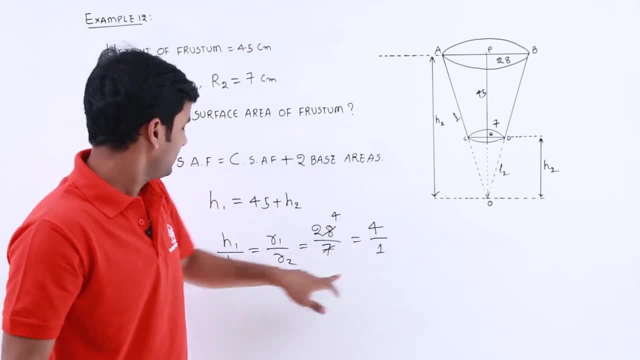 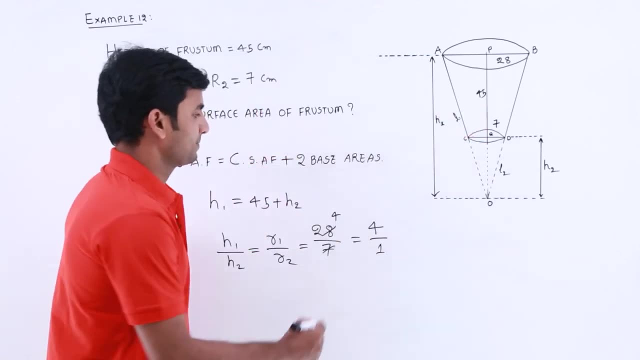 So complete height of cone is 4 parts. So this H2 is one part of this complete H1. So here the remaining 45 is 3 parts. So here 3 parts become 45. Then what about the one part? 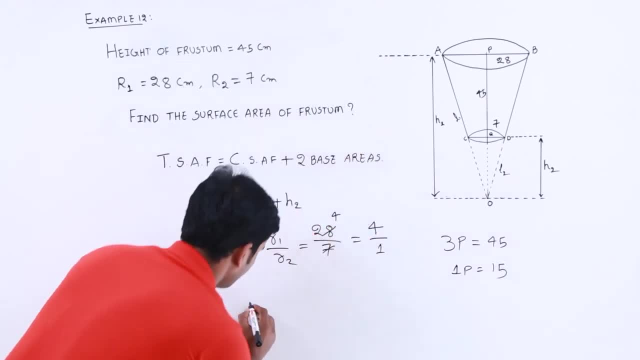 That will become 15.. So here the H1 value will be No H2 value will be 15 centimetre. If you substitute this H2 into this H1 equation, we will get H1 as a 60 centimetre. 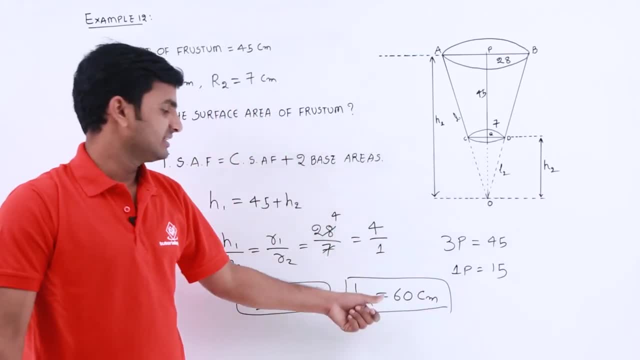 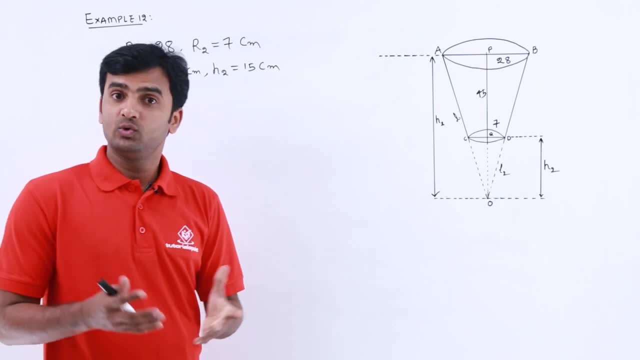 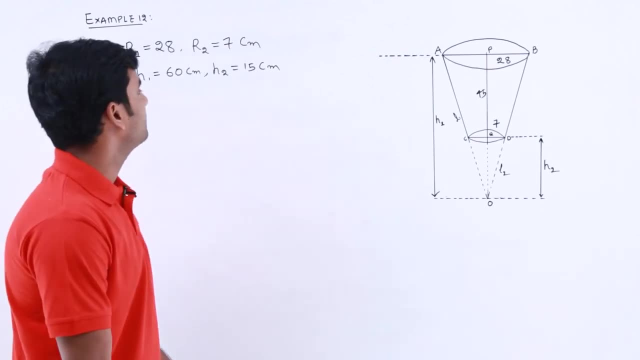 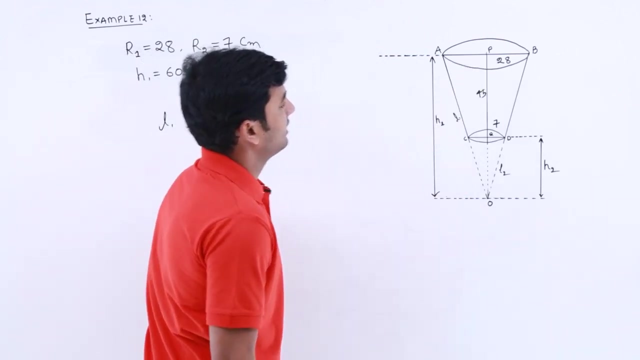 value of R1, R2 and H1- H2.. To find out the curved surface area of cone, formula will be pi, RL. Here we do not know the value of L here. So here we have to find out value of L1 and L2.. Here the L1 will be. if you observe triangle OAP, it looks like a right. 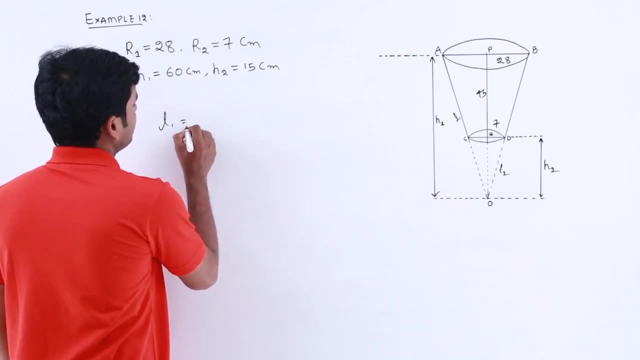 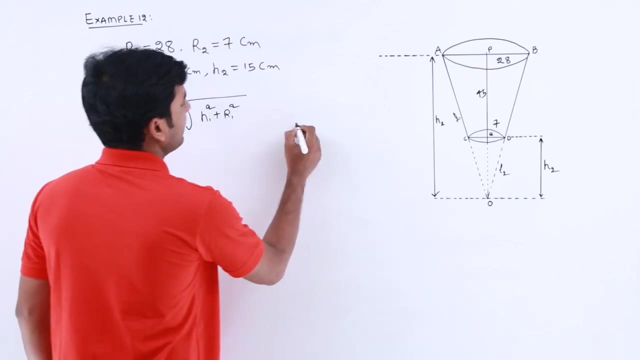 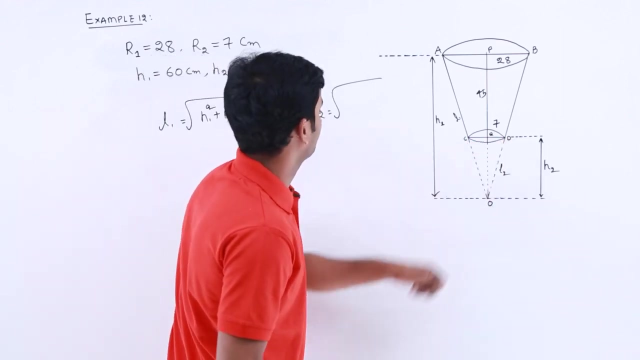 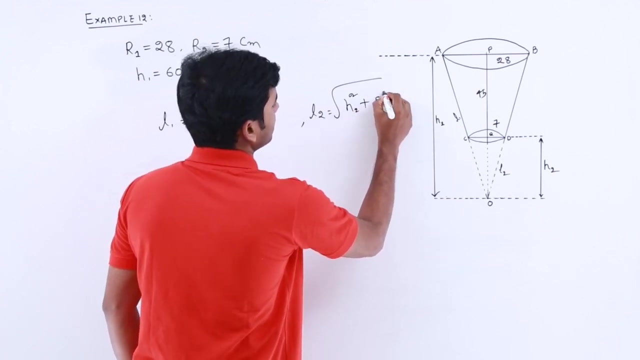 angle triangle. We can use Pythagoras theorem here. L1 is equal to under root of H1 square plus R1 square and L2 will be triangle OQD, that is, H2 square plus R2 square. If you substitute these values, we will get L1 plus R2 square. 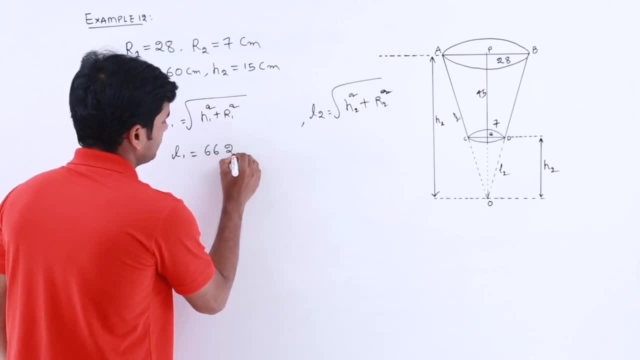 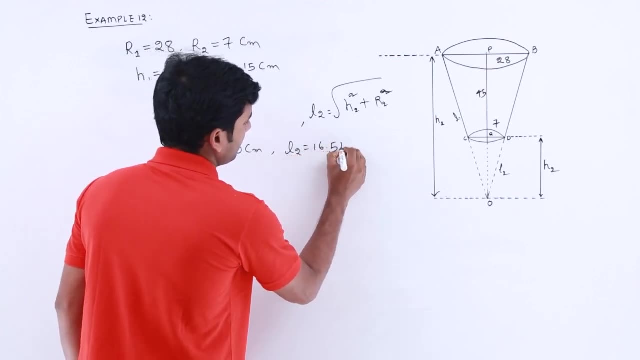 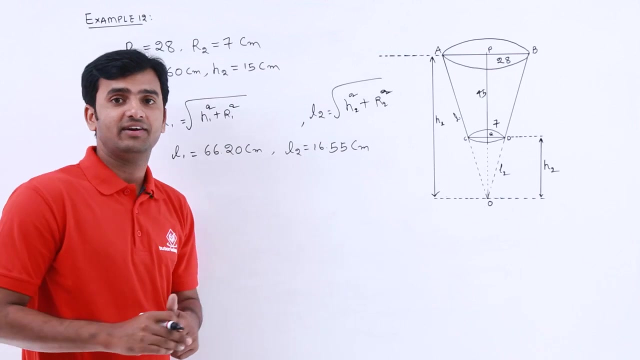 So L1 will be as 66.20 centimeter and L2 will be 16.55 centimeter. So now we know R, H and L values, we can easily find out the curved surface area of cone. Here we 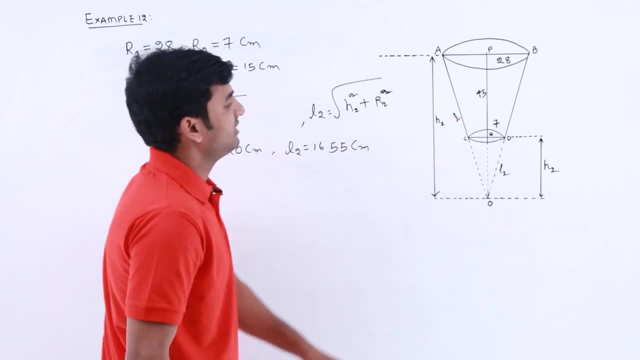 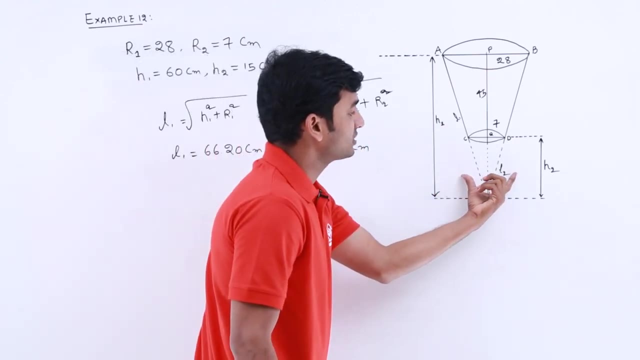 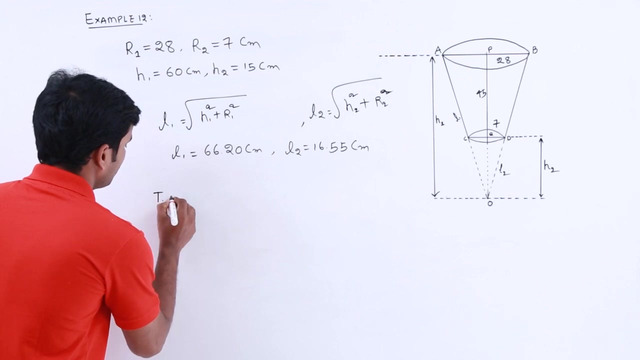 have to find out the curved surface area of frustum. So for that we have to find out the complete cone surface curved surface area And we have to subtract the extended portion cone curved surface area. then we will get frustum curved surface area. So that will be the total curved surface area of frustum. 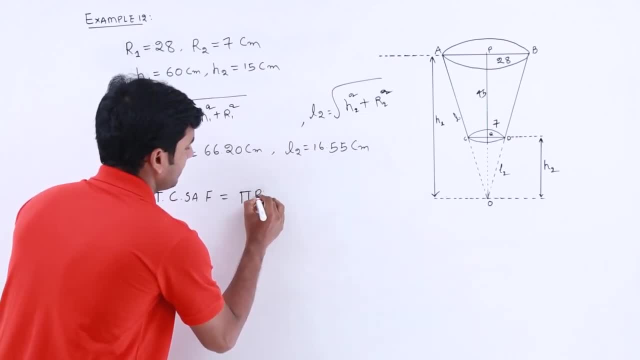 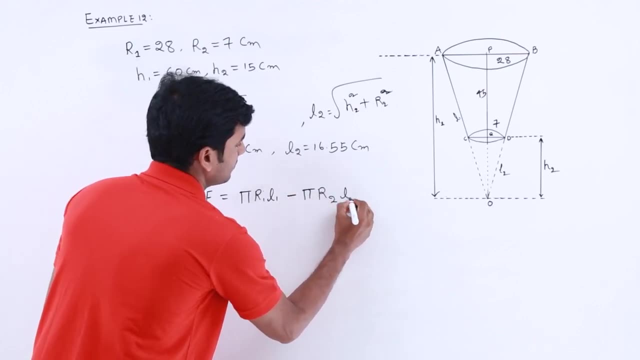 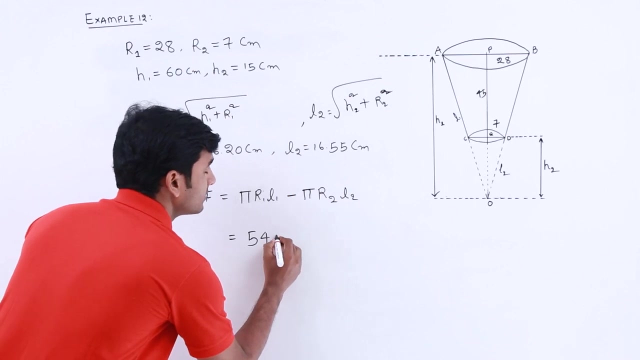 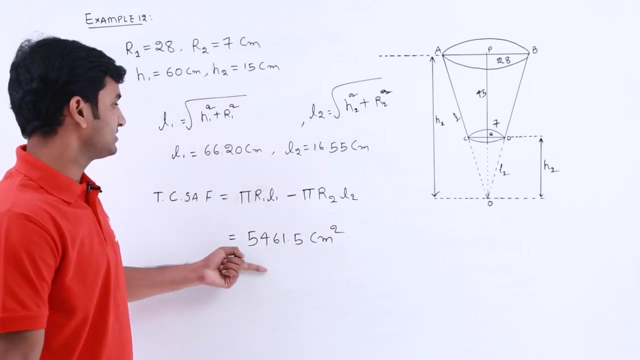 is equal to pi R1 and L1 minus pi R2 and L2.. If you substitute values, we will get phi 4, 61.5 centimeter square. So this is the curved surface area of frustum. But we have. 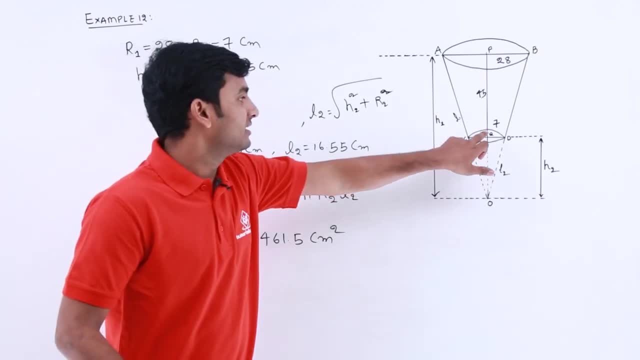 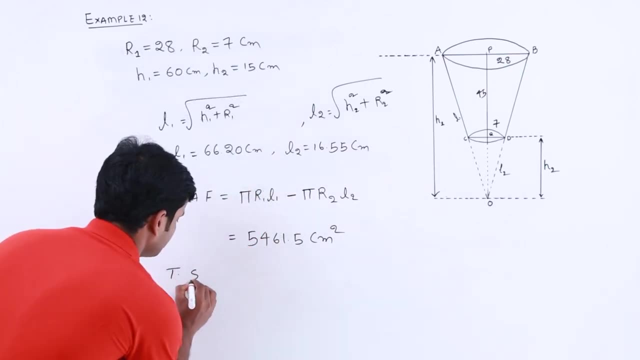 to find out the total surface area of frustum that is included these two base circular areas also Here. the total surface area of frustum will be phi 4, 61.5 plus L2.. So this is the total surface area of frustum. 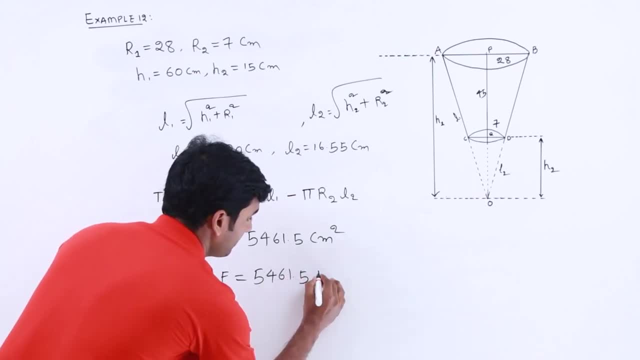 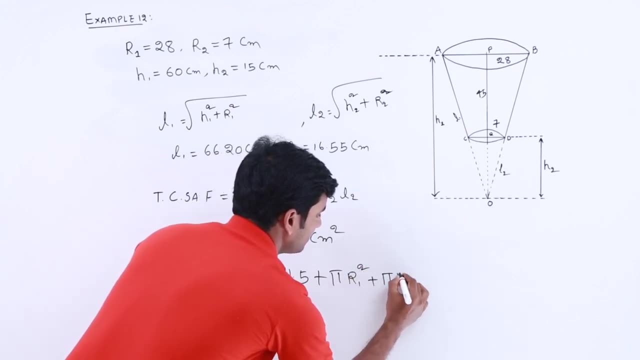 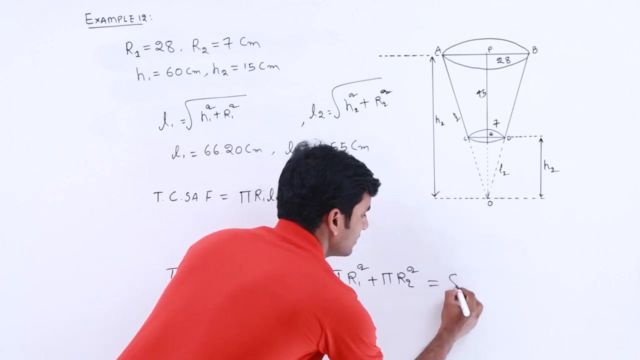 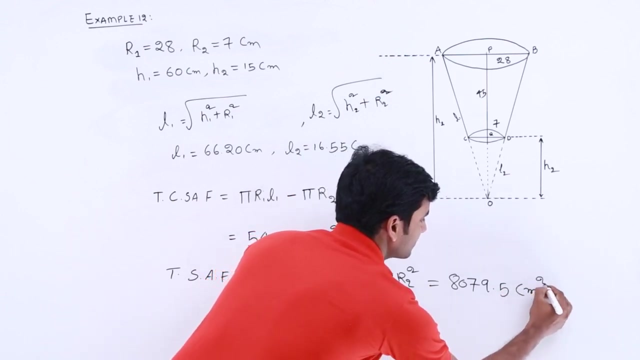 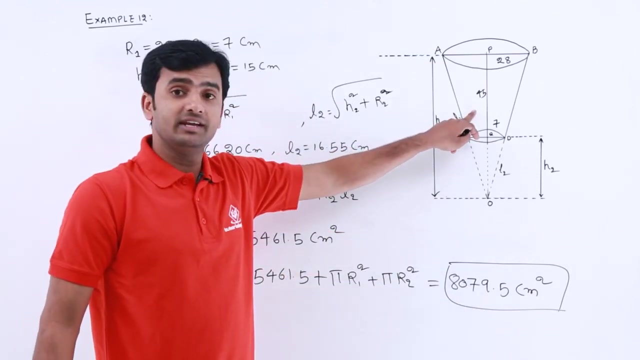 So this is the total surface area of frustum. Number of slabs will be phi 5 plus phi R1 square plus phi R2 square. If you substitute R1 and R2 here, we will get 8079.5 centimeter square. So this will be the curved surface.